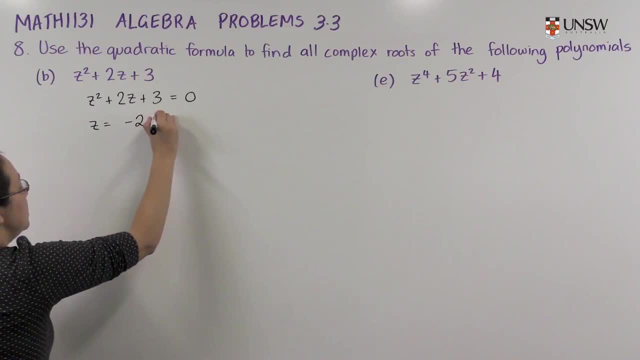 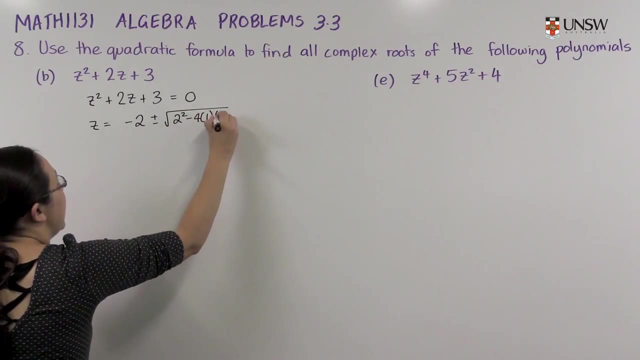 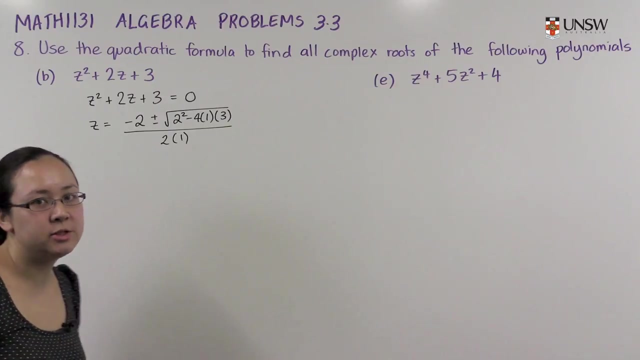 do So, z will equal minus b, plus or minus the square root of b, squared minus 4ac, All over 2a. So we're just substituting into the quadratic formula. You can complete the square to solve this quadratic. you don't have to use the quadratic formula here if you don't want to, But if 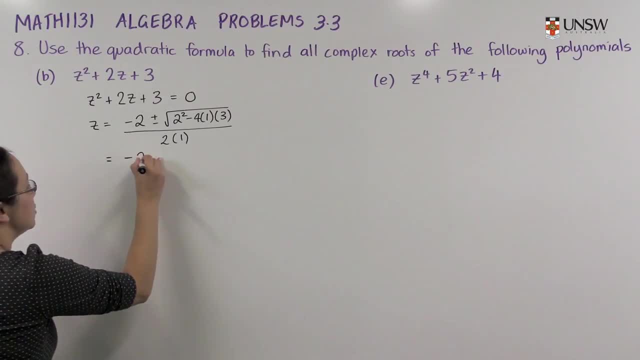 we simplify: here we'll get minus 2, plus or minus the square root. Now here we'll have 4 minus 12.. So that's negative 8 all over 2.. Now the square root of minus áreas isn't a real number. we can't square root negatives to get a real number, but it is. 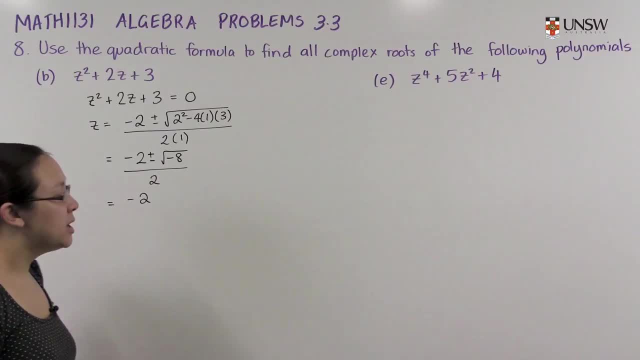 a complex number and we can simplify it. So the square root of minus 8 is the square root of 8 times the square root of minus 1.. The square root of minus 1 is just i, and the square root of 8 simplifies to 2 root 2.. So here we have 2 root 2 for the square root. 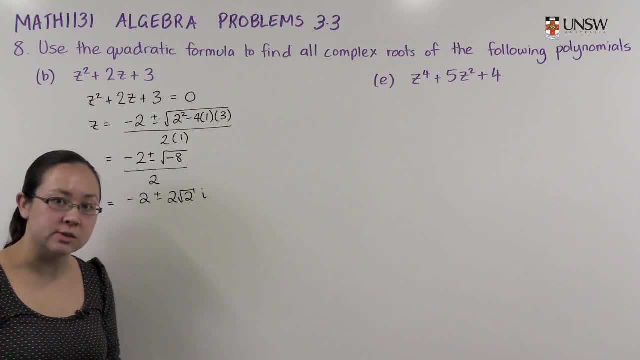 of 8, and we have i for the square root of minus 1.. So we're just simplifying here all over 2.. So this gives us dividing everything by 2 here, minus 1, plus or minus the square root of 2i. So these are the complex roots of this quadratic here. So therefore minus. 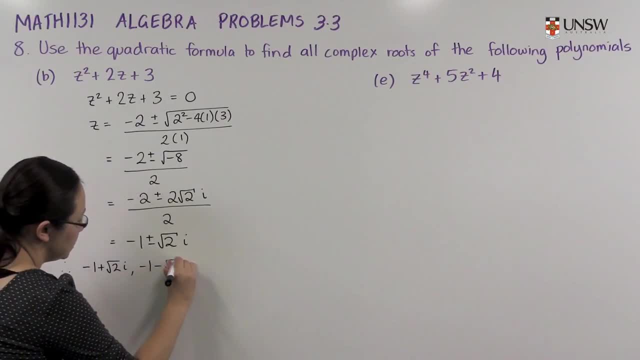 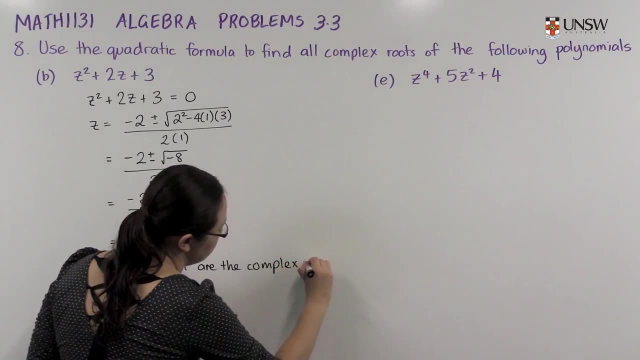 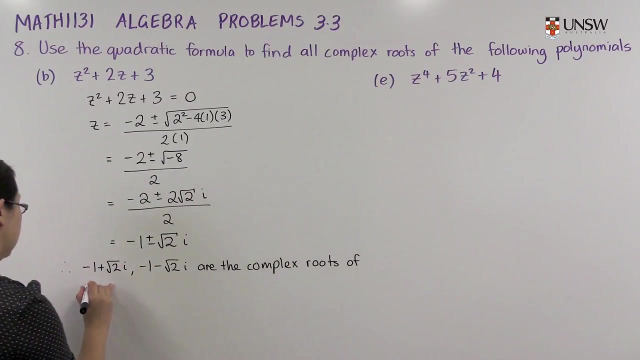 1 plus root 2i minus 1 minus root 2i are the complex roots of z squared plus 2z plus 3.. Okay, so that's the answer to our question, but there's a couple of things that we should notice here. The first thing we should notice is that the 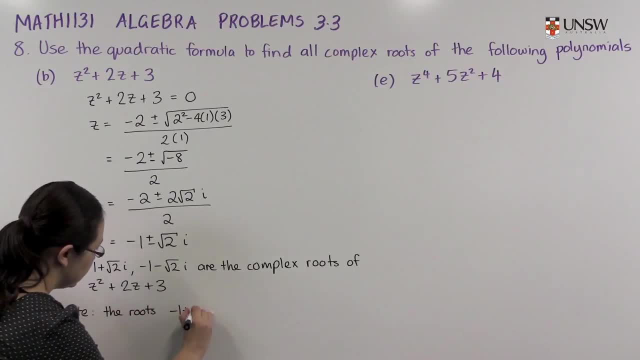 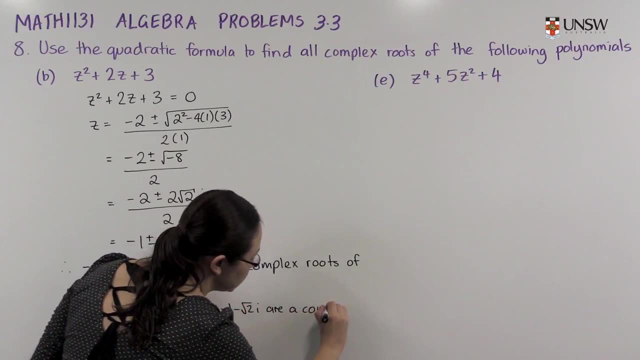 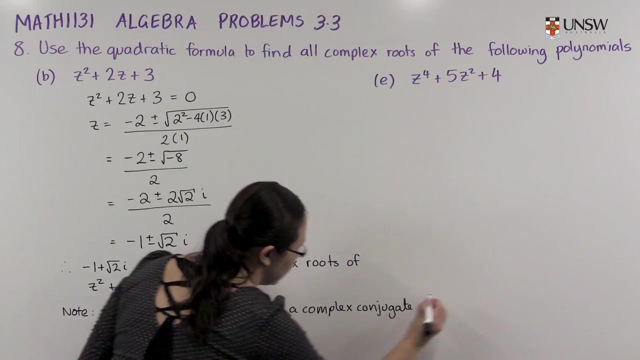 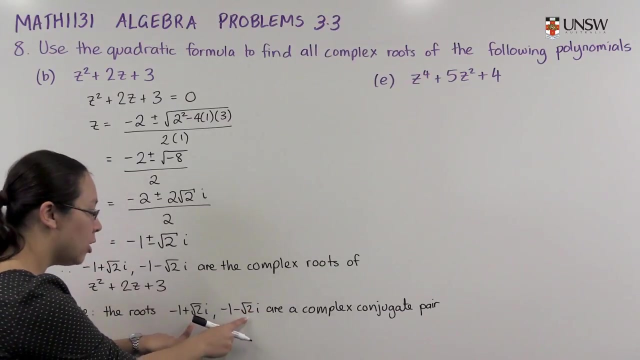 roots. so these roots here are a complex conjugate pair. Okay, this is minus 1 plus square root 2i. this is minus 1 subtract square root 2i. So these are complex conjugates here. right, That will always happen. 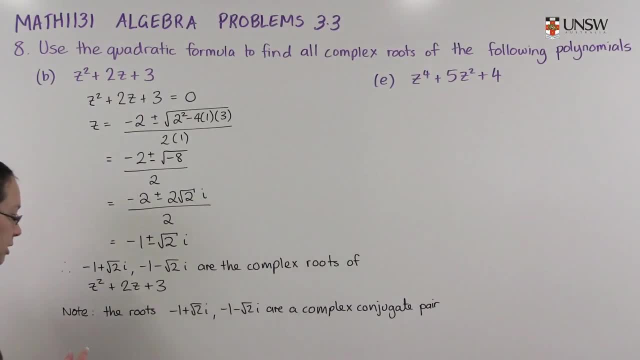 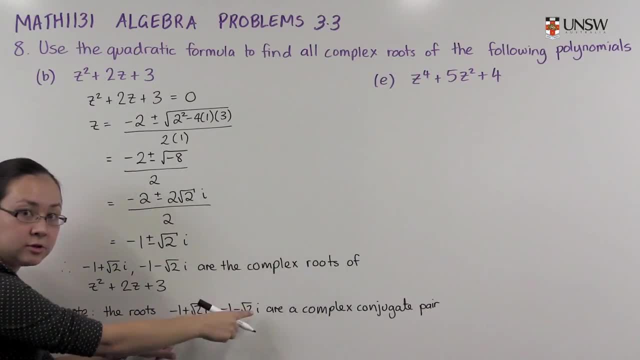 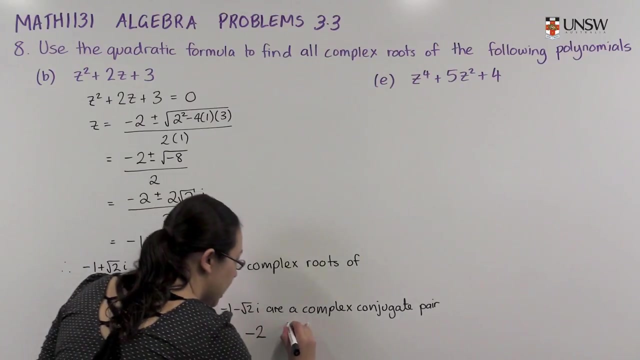 so if I add these two roots together here, minus 1 and minus 1 gives me minus 2 and plus root 2i. minus root 2i gives me no imaginary part at all. so the sum of the roots is minus 2.. First of, 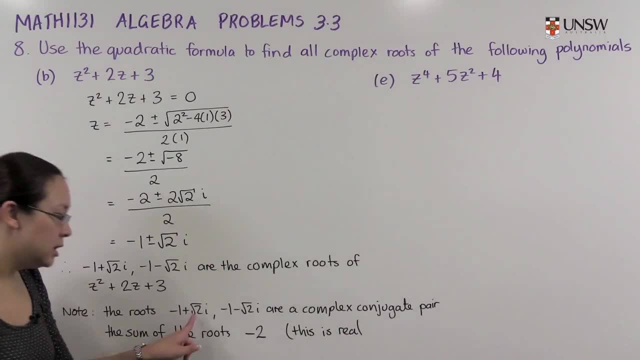 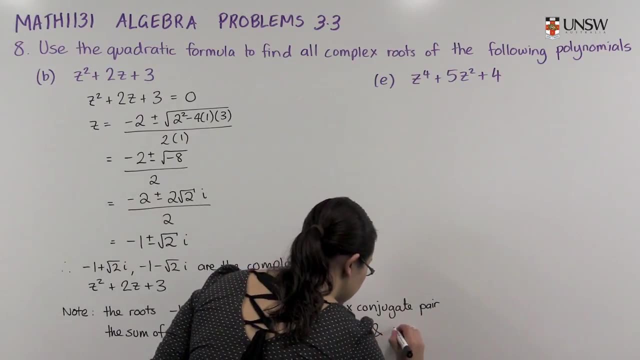 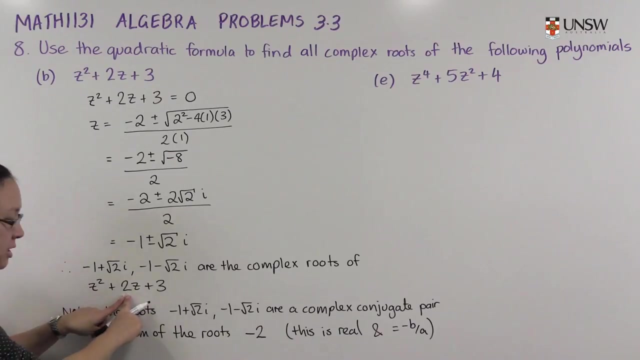 all, it's real, okay. the complex, the imaginary parts, went away. they added to 0 and no, it equals minus b on a right. We know the sum of the roots should be minus the coefficient here divided by the coefficient here. so that should be what. 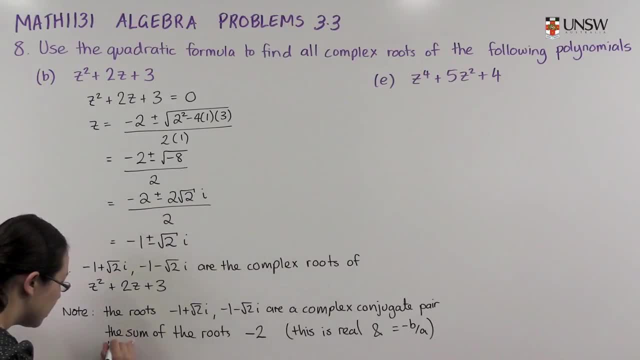 we expect. Lastly, the product of the roots, I should put an is there is. so if we multiply these roots here, we actually get to have a difference. of two squares: We have minus one. it's a because it's there in complex conjugates. it's minus. 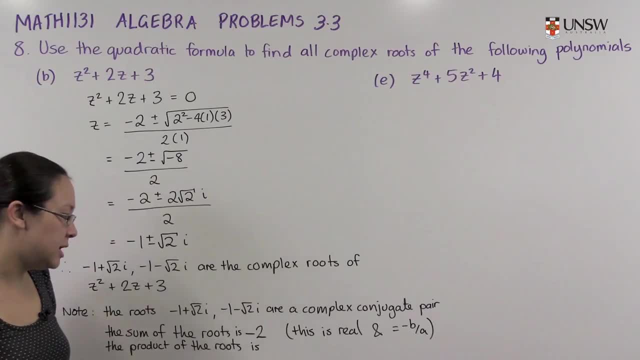 one plus root two. i minus one minus root two. i. we can expand. it's a difference of two squares. so it's minus one squared, which is one subtract root two. i all squared. so that's one minus two, i squared, or one plus two, which is three. 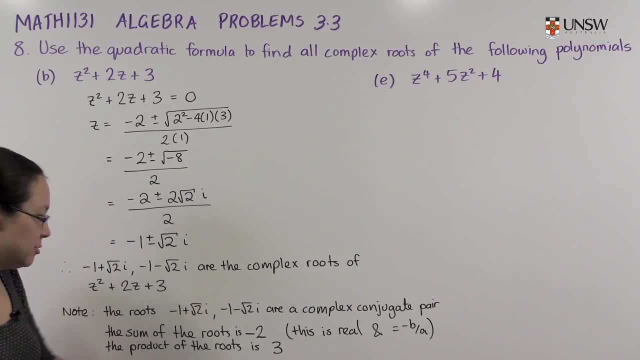 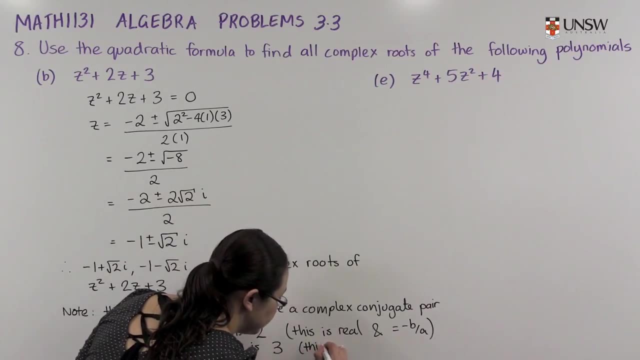 Okay, so I'm just running out of room, so I'm not putting the working, but when you multiply these out, you will get three. So, again, this is real. Okay, the imaginary parts went away because they ended up being a. 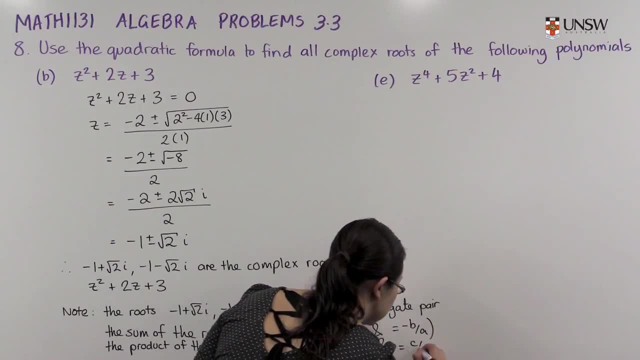 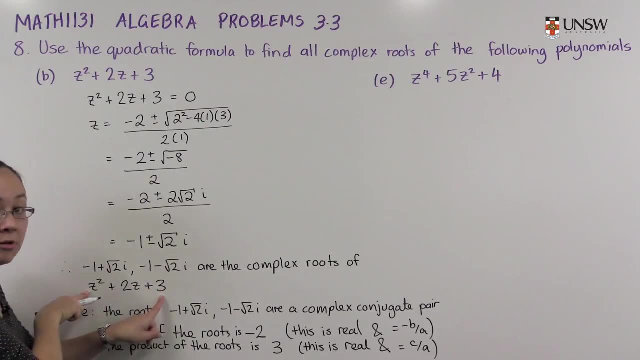 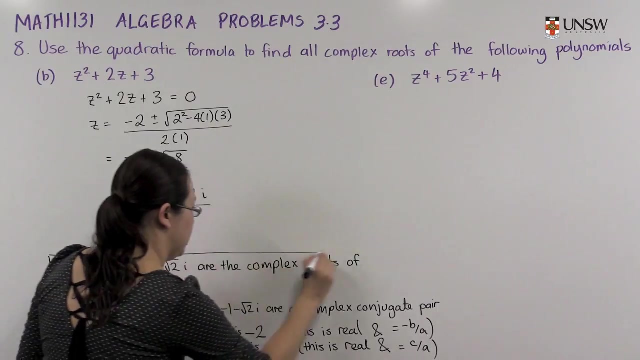 difference of two squares and furthermore it equals c on a. It should be what it we expect. so this polynomial here, three divided by one right, is the product of the roots. So your answer is here, but these other facts that I've written down the bottom are important things to 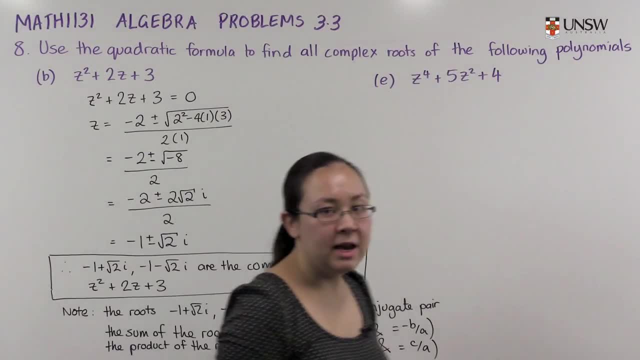 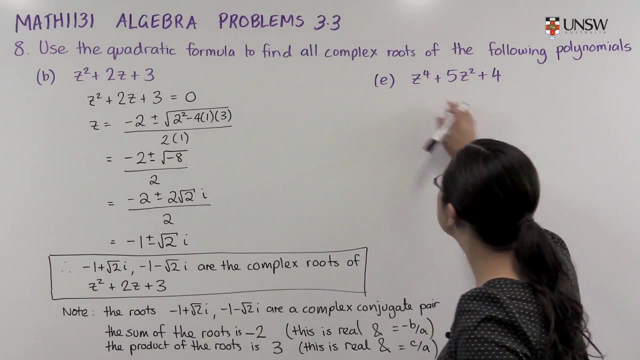 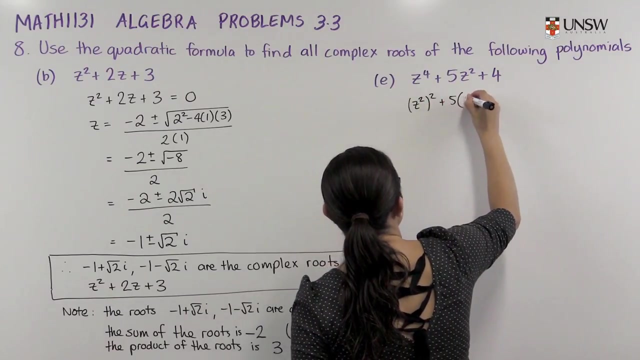 realise, Going on to part e, we don't have a quadratic here, we have a quartic, but this quartic is really a quadratic in disguise. Okay, this quartic really looks like a z squared being squared. five, lots of a z squared plus a four. Okay, now we're trying to find 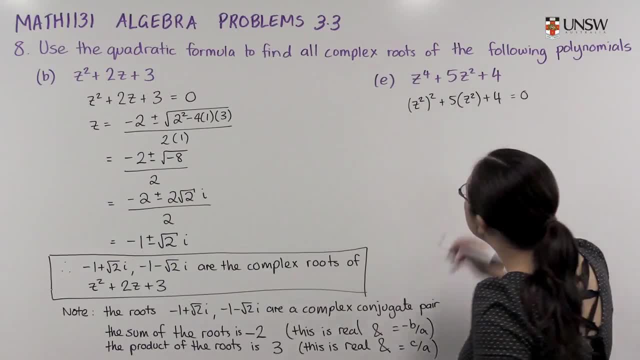 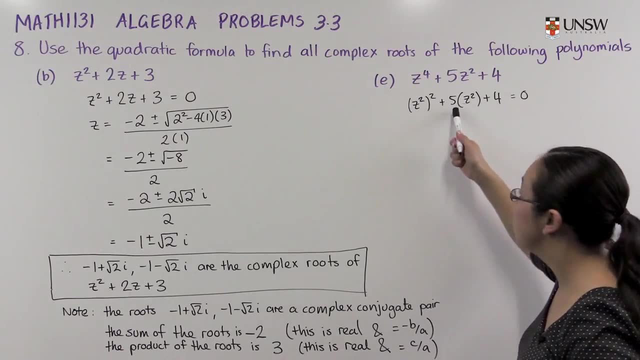 the roots of these. so we're trying to solve this. equals zero. Now you could use the quadratic formula to solve this, but we can actually factorise it because I can find two numbers that multiply to four and add to five. they're four and one. So this actually factorises and that turns out. 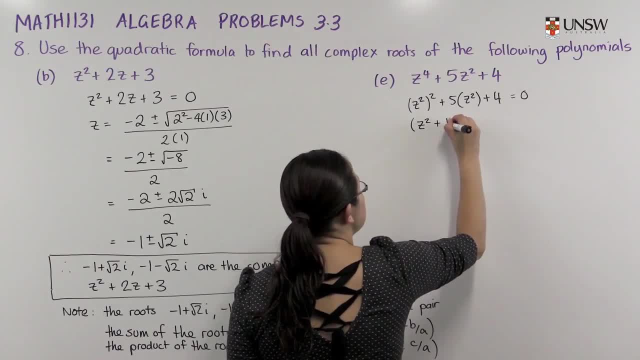 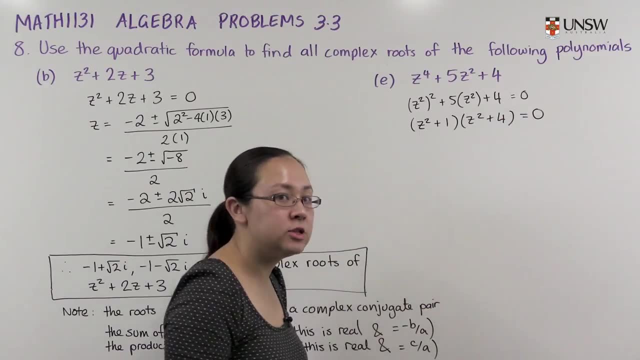 to be much easier, I think. So let's factorise it into z squared plus one. z squared plus four is equal to zero. You can always double check. that's correct. this expands to z, to the four plus four. z squared plus one. z squared is five z. 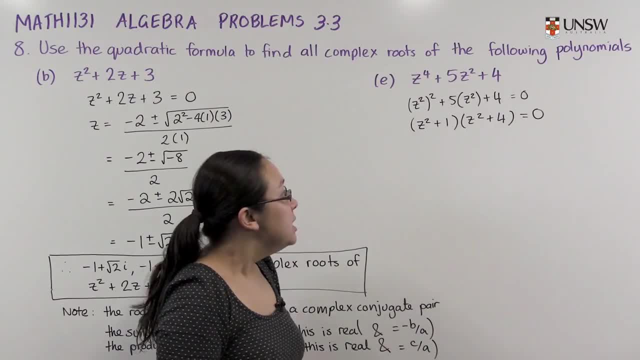 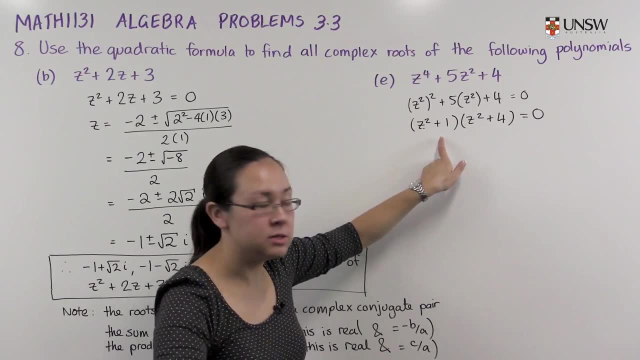 squared plus four gives me four. Okay, now I could say from this point: if these two things multiply to give zero, z squared plus one is zero, or z squared is minus one, z squared plus four is zero or z squared is minus four. I can solve it like: 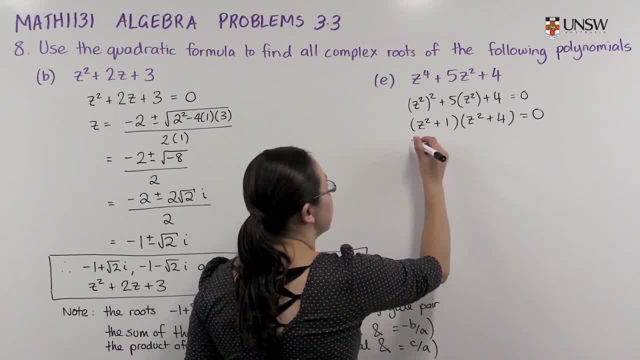 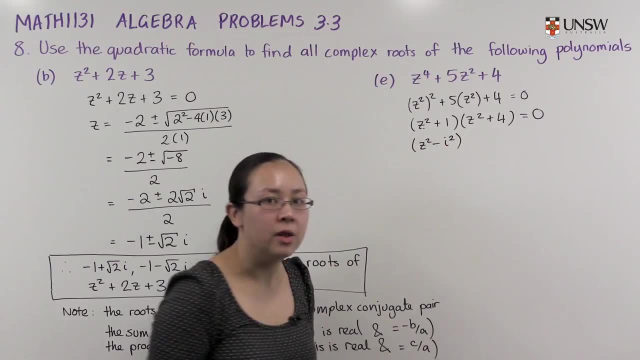 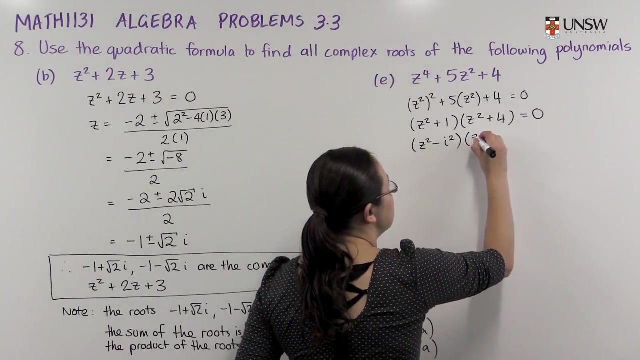 that, but I'm actually going to factorise here just because I can. So z squared plus one is actually z squared minus i squared i squared is minus one. so minus i squared is plus one. Similarly, z squared plus four is z squared. 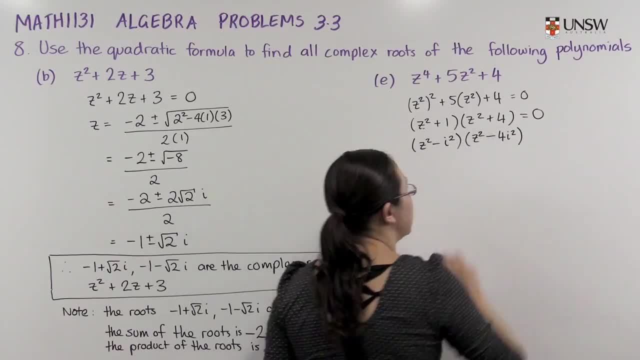 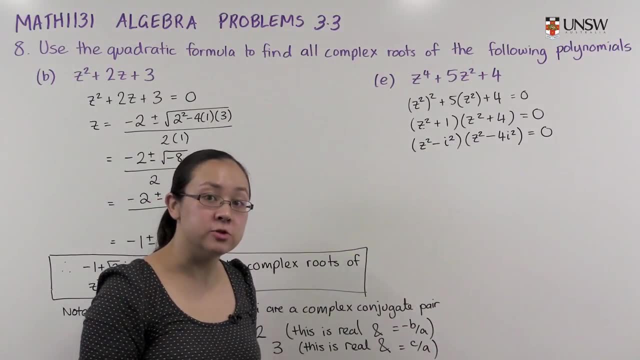 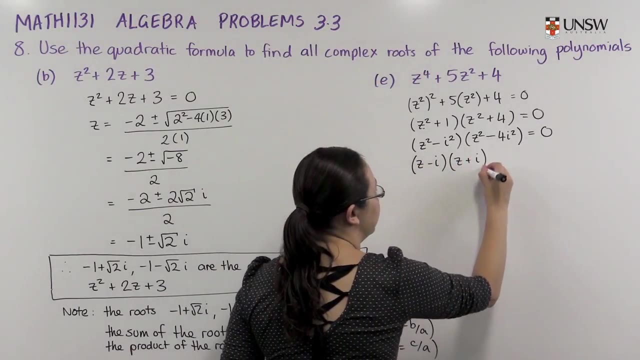 minus four, i squared. Okay. and the reason I want to do that is because now z squared minus i squared is a difference of two squares and I can factorise it. So this gives me z minus i times z plus i. and the second factor here gives me z minus two, i z. 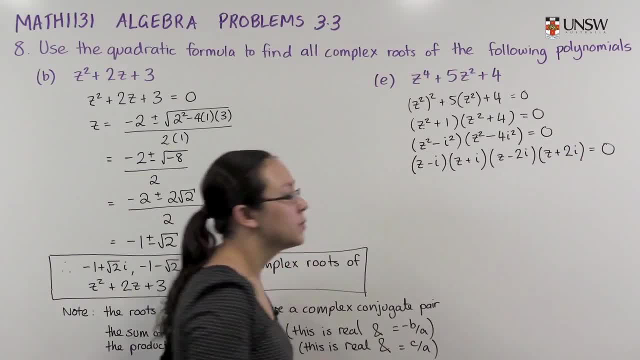 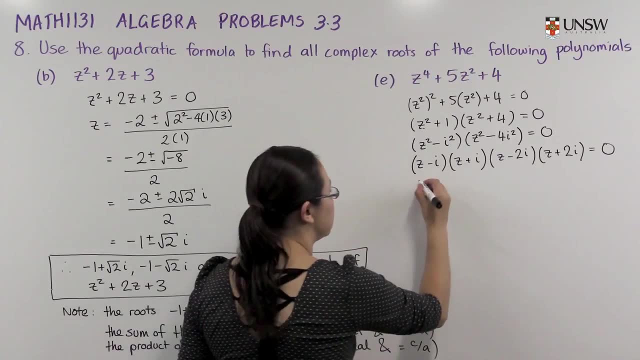 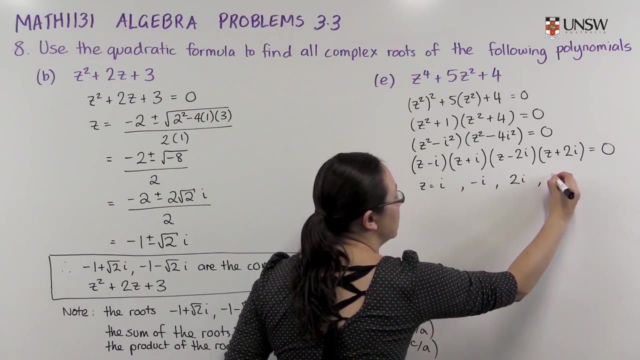 plus two i. Okay, and from here I can write down all my roots. So four things multiply to give zero. one of them's got to be zero. so either z equals i or minus i, or two i or minus two. i Notice again they come in complex conjugate pairs.